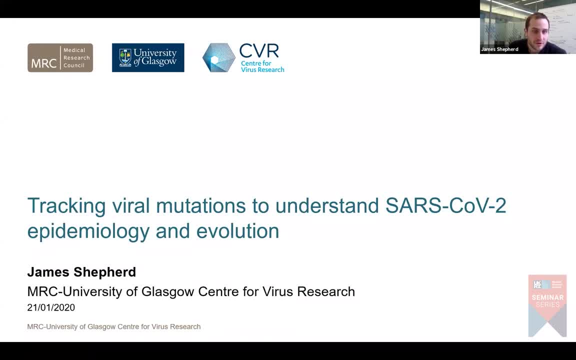 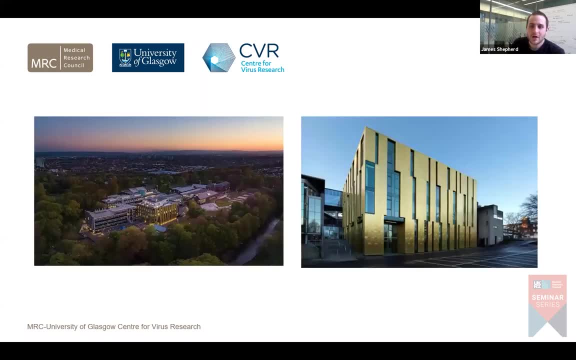 here on sequencing SARS-CoV-2 as part of the response to the COVID-19 pandemic. So I work here at the Centre for Virus Research, which is an MRC-funded virology research institute which is hosted at the University of Glasgow and we're based on this nice campus just on. 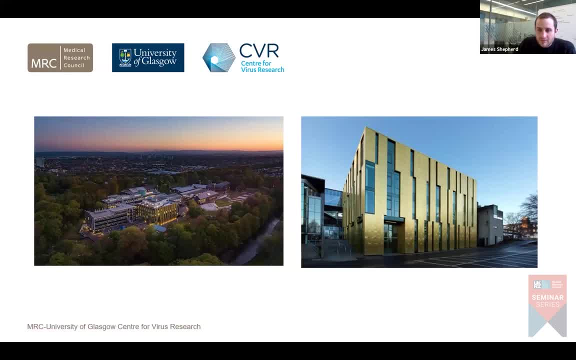 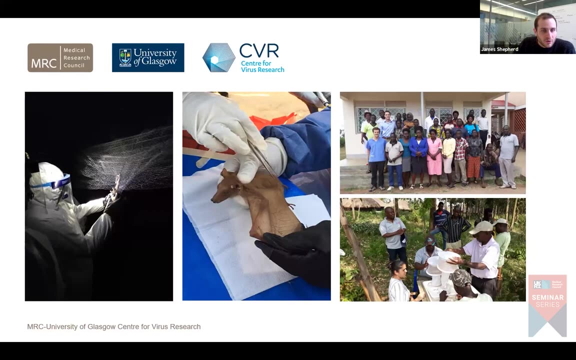 the outskirts of Glasgow And I've been a. I've been lucky enough to benefit from MRC funding, which has enabled me to take three years out of my clinical training to study virology, And my interests were before the pandemic, were in emerging viruses such as SARS-CoV-2, and my research was focused on. 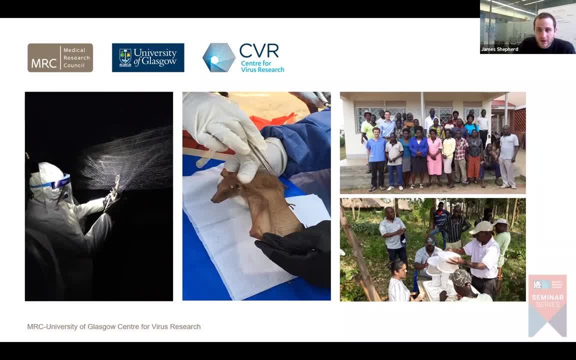 emerging viruses in Uganda using a technology called next-generation sequencing, And to do that we were. we set up a clinical study at a site in northern Uganda where we did blood samples from patients presenting with unidentified acute Marblekan virus virusbres and then used this technique to detect viruses that might be causing them to become unwell. 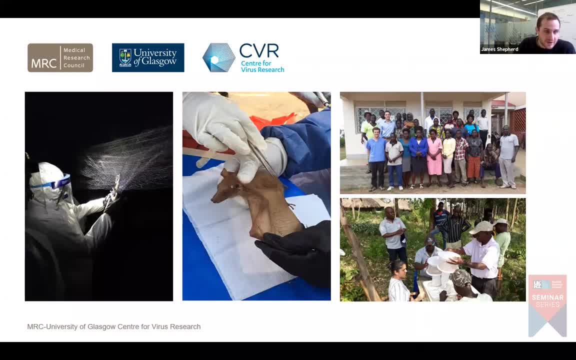 And we were interested in what was causing people to become unwell. but we're also interested in the animal viruses And the things that might be spilling over from the local wildlife. So we also sample, did ecological sampling, And that included wildlife such as bats. linha olmuşishoes bay, contrib occas. So we also stuffed ourselves to do ecological sampling, and that included wildlife such as bats. 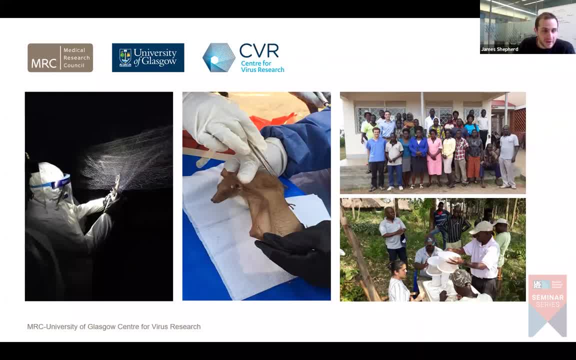 and that included wildlife such as bats And weri cafes- and we are called up to the- And that included wildlife such as bats, rodents, collected mosquitoes and also livestock. So I had some experience of emerging viruses and the use of sequencing technologies to detect them. 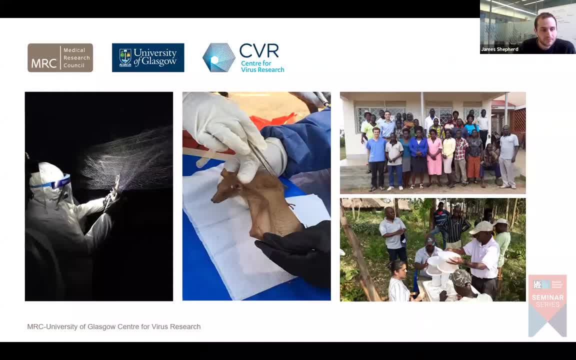 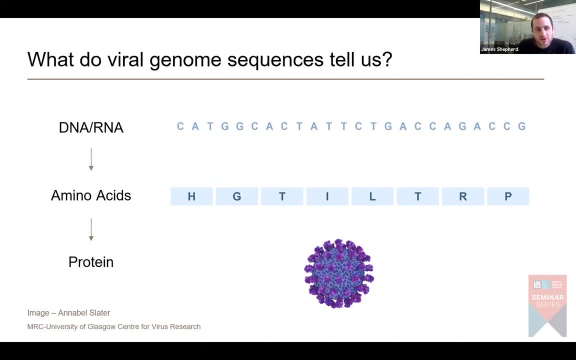 prior to COVID-19.. So just to make clear what the viral genome sequences can tell us. so a genome sequence is made of four nucleotide bases that code for amino acids, which are the building blocks of proteins. So if you understand the genome or the genomic sequence, 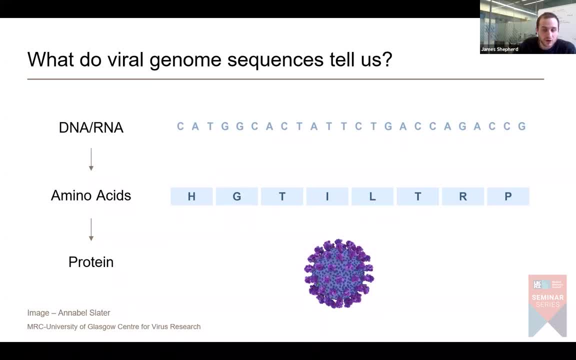 of an organism, such as a virus or humans or bacteria. we're able to see what amino acids are made and then we're able to have a good understanding of what proteins that organism makes. So it tells us the instructions, the instructions for how to make the virus. 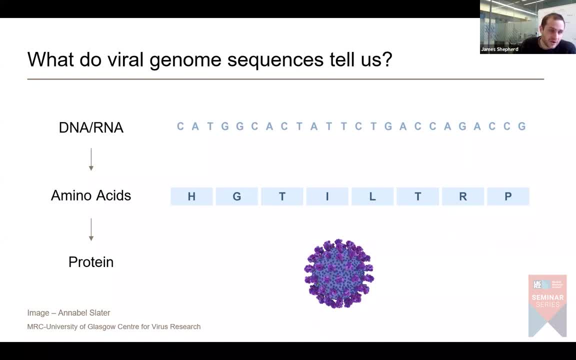 and it enables us to understand how it works. The flow of information goes from the genome sequence to amino acids and then to protein, and this is a visual representation of SARS-CoV-2.. And, for example, these knobbly bits on the outside: 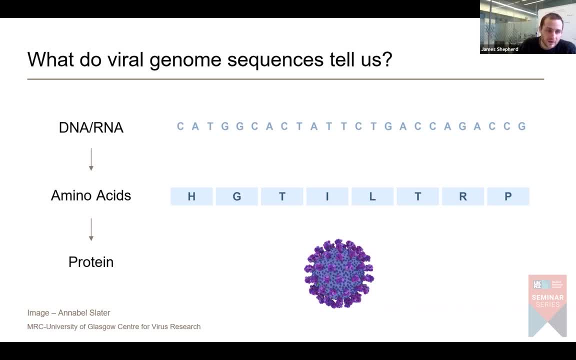 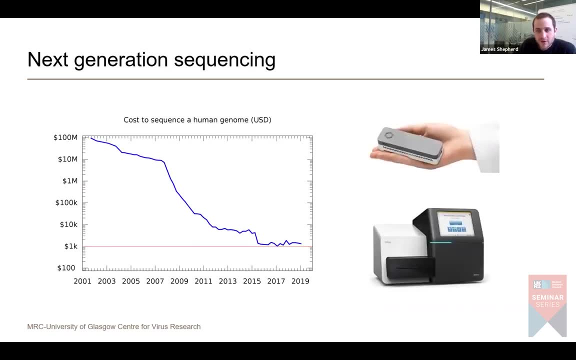 are the spike protein and these are coded for by amino acids and the DNA genome sequence. So over the last 20 years, generating genome sequences from humans or bacteria or from viruses has become a lot easier because of the advances in sequencing technology. 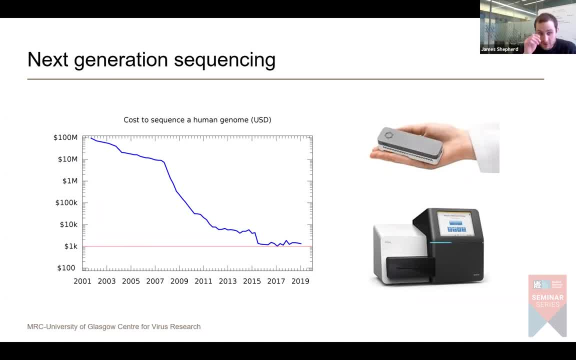 that enable us to generate whole genomes from pretty much any biological material much faster and at a much cheaper cost than it used to be. So if you look back at about 2001,, when the Human Genome Project was in full swing, they were using older technologies. 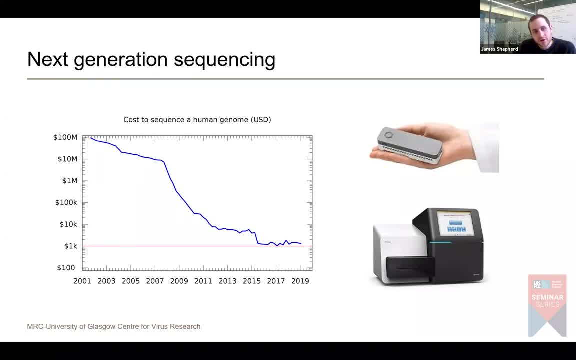 such as cybersecurity, but over the next 20 years. new technologies from companies such as Illumina and Oxford Nanopore have meant that this can happen a lot more quickly and the cost is a lot less. And that's not just had implications. 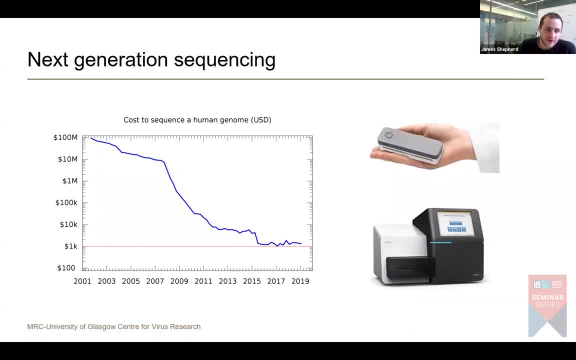 for human genomic research, but it's also still going to pathogen genomic research, And these technologies are called next generation sequencing just because of the advances that they give over previous methods in speed and cost, As an example back in 2009,. 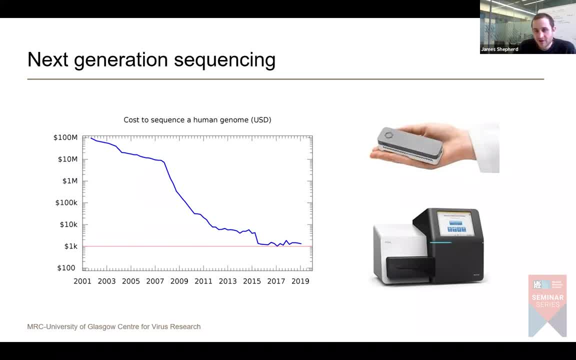 there was a study that was done in the United States of America and it was called Next Generation Sequencing, and it was a study that was done in the United States of America and it was called Next Generation Sequencing and it was a study that was done. 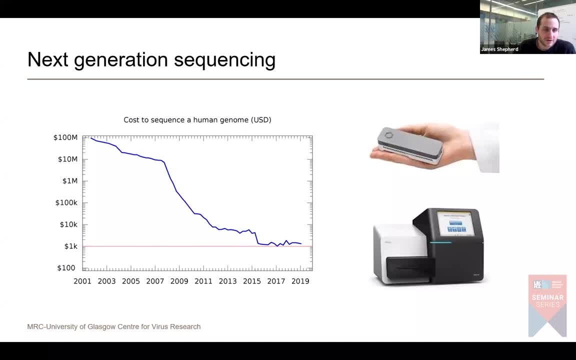 in the United States of America and it was a study that was done in the United States of America that the traditional genome sequencing for genomic gene sequencing had many investment reverse taxes on… On this occasion, when the virus emerged in December 2019,. 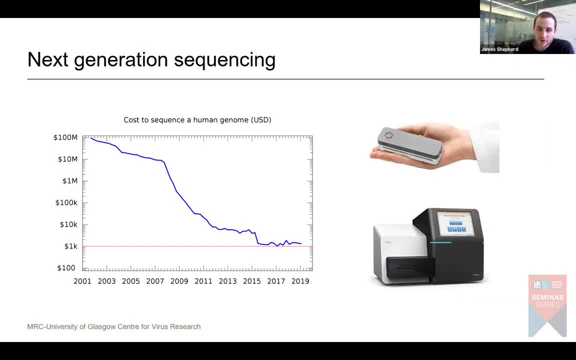 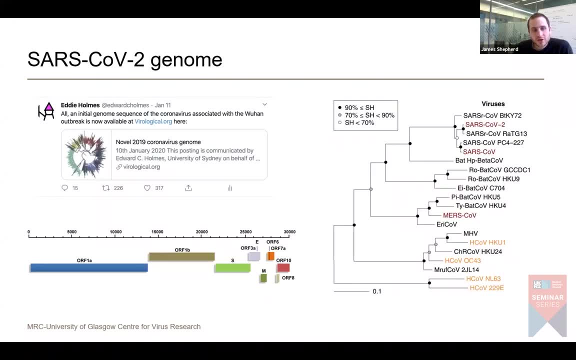 by the start of January, the virus that causes COVID. So we're really benefiting from this technology. So the initial genome of SARS-CoV-2 was shared online on the 11th of January and because the genome contains the instructions for creating the virus and for the proteins, it 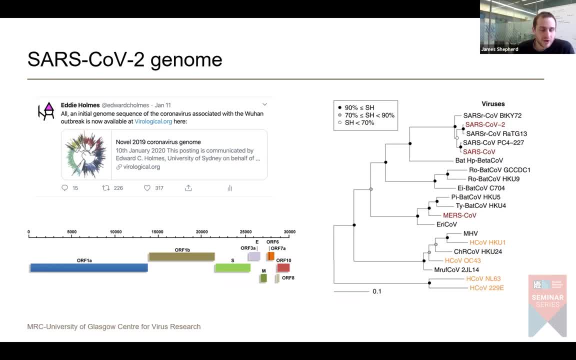 produces. researchers were able to right away look at this genome sequence and begin to generate response to the epidemic, such as vaccines. So once they had that genome sequence, that allowed vaccines and other countermeasure development to start right away And the genome sequence showed that we were dealing with the coronavirus. It was very similar. 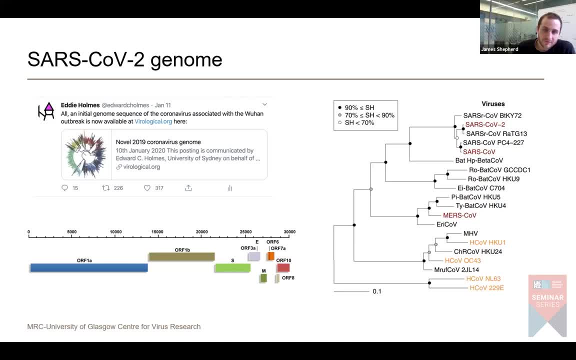 to the initial SARS-CoV-2. So this is an evolutionary tree called the phylogeny. Once we have the genome, we can compare the genome to the genome from other viruses and see where our SARS coronavirus genome fits into the kind of viral 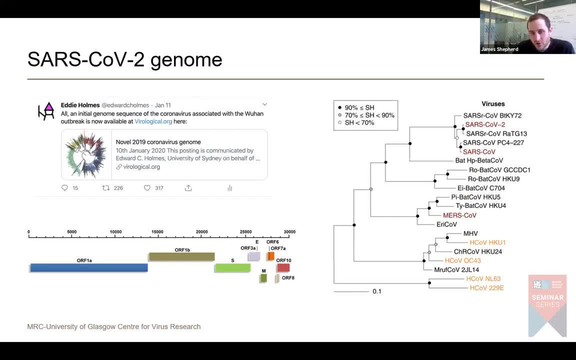 tree of life, and so this phylogeny is showing that SARS called two groups very closely with some bat coronaviruses. so that gave us an idea that it probably spilled over from a bat reservoir. and then it's also quite close to the original SARS virus, so that gave us a warning shot that. 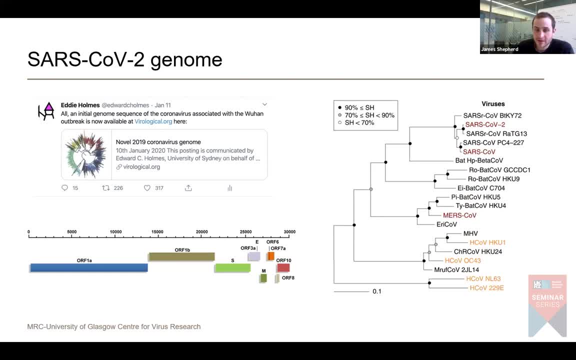 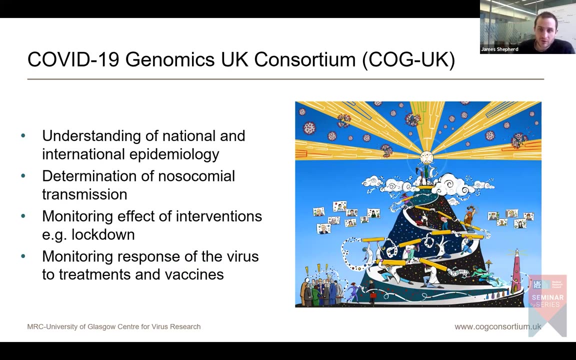 this might be something spread from person to person and cause people to become unwell. Because I had experience in next generation sequencing from my PhD project prior to COVID, I was redeployed to work on COVID-19 genomics rather than being redeployed back to the hospital. 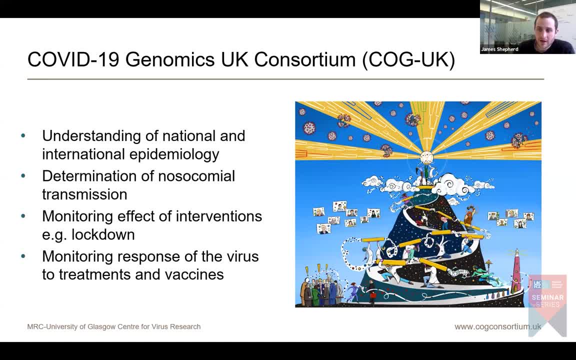 like a lot of my clinical research colleagues were, and by March it was becoming pretty clear that you know that a pandemic was underway that was going to come to the UK and it was going to be quite significant. so in response to this, this COVID-19 genomics UK consortium was set up and that was funded by UKRI. 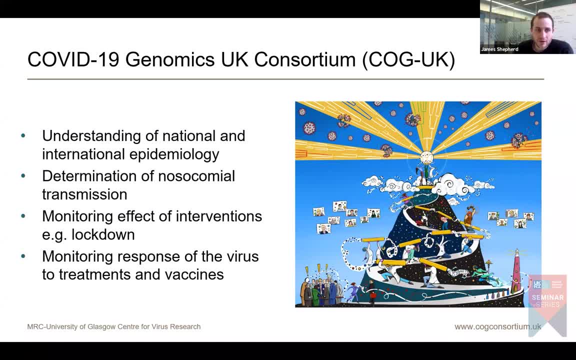 and also some funding from Wellcome, the Department of Health and Social Care, and from the Sanger Institute, and the goal was- these were the goals really- to understand the national and international epidemiology of COVID-19 and to determine nosocomial. 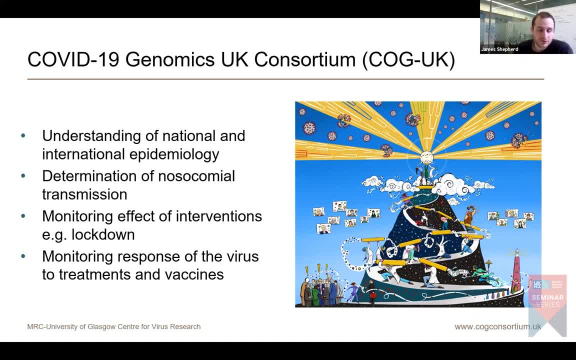 or hospital or healthcare associated transmission, to monitor the effects of interventions on the virus genome, such as lockdown or vaccines and other treatments, such as drug treatments like erythesivir convalescent plasma, and these goals were all hopefully to be achieved by performing large-scale genome sequencing from COVID-positive patients in the UK. 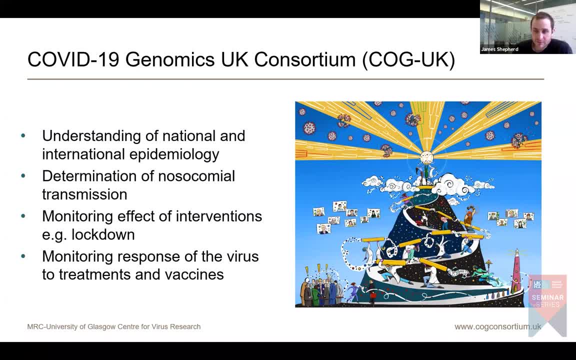 This brought together multiple academic partners and NHS partners from across the UK and it's actually been very successful. so since we started in March, we've generated over 200,000 genomes- whole genome sequences of COVID- from individuals that were affected in the UK and that 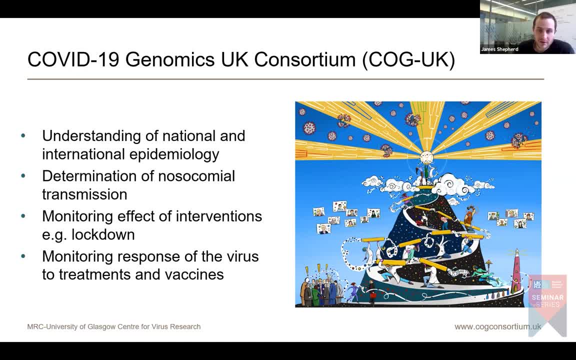 gives us a kind of unparalleled understanding as to how the pandemic has unfolded and how the virus is spreading. And lastly, I should say that all that data is provided open access, so researchers anywhere in the world are able to access that data And they can access the genome sequences that they're producing and they can use them for analysis. 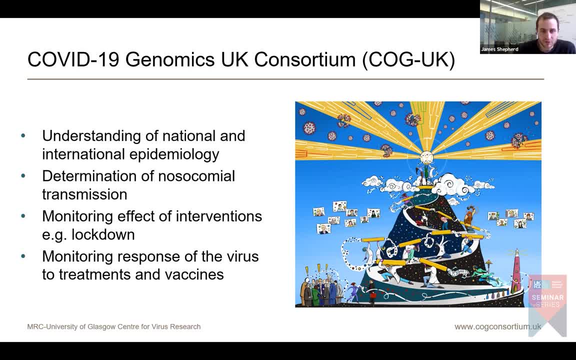 so kind of generate this data, but anyone across the world can use it at open access. This is just some artwork from an article that's on the COG website describing the process that we've gone through to get it set up. so if people are interested in COG, I would 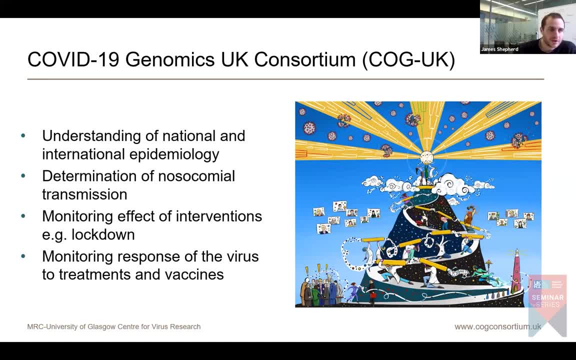 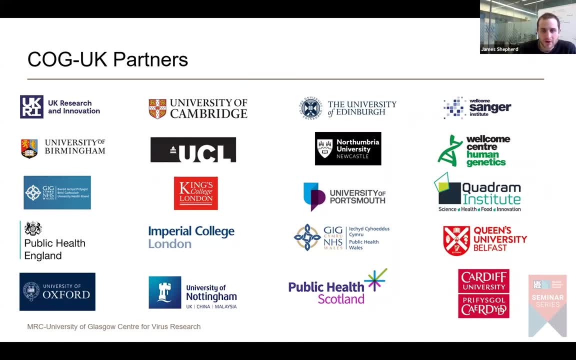 recommend you go to the website and have a look and read some of the articles there, And these are just some of the partners that that were there at the start of COG, and there's many other partners joined over the last 10 months, but it really does. there's partners from right across the UK. 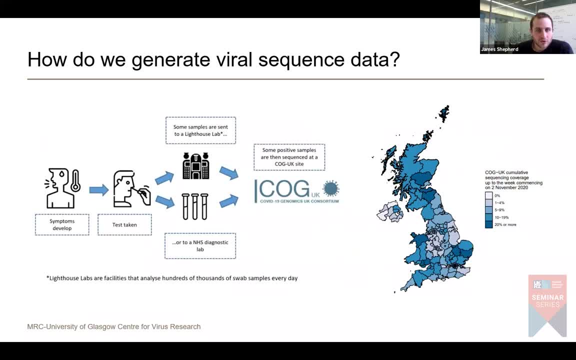 So how do we generate viral sequence data or whole genome sequences? So it all starts with a patient who comes unwell, develops symptoms and will these days, will arrange for a COVID-19 test to be taken. So when you go for your test, you'll have a. 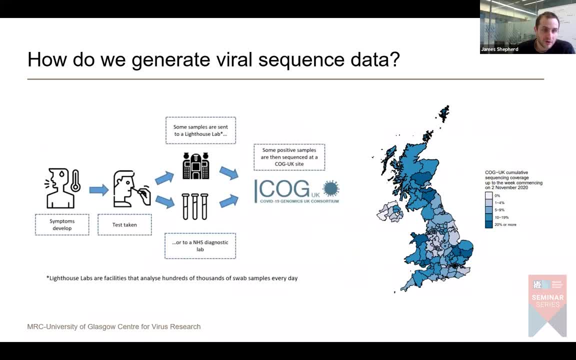 swab and that will be sent to one of the large kind of mega labs, these lighthouse labs or an NHS diagnostic lab, and that will be tested using a PCR test which is there to detect virus genetic material in that sample and if it's positive it's because we've detected virus RNA there. 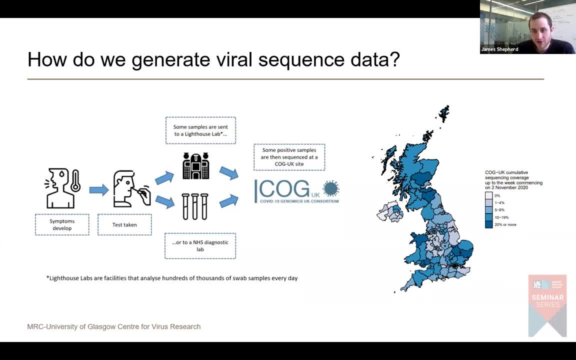 So a proportion of these samples containing virus and the viral genome are then sent to a COG UK site, such as here at the Central River. And this is just a map demonstrating the proportion of positive sequences. positive samples, sorry, that have been sequenced at various locations across the UK and it's a bit 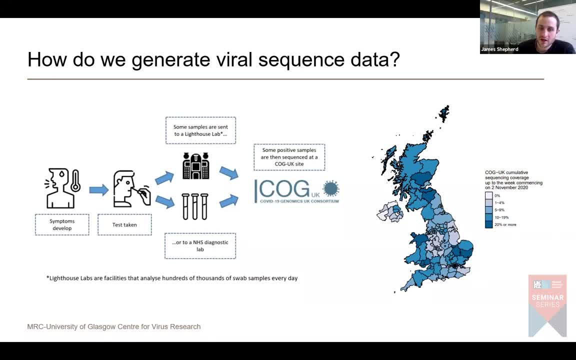 patchy just because of the volume of positive tests and the sequencing capacity there. But overall we sequenced about between about 10 percent of all positive PCR tests in the UK. So this is just a map demonstrating the proportion of positive samples that have been sequenced at. 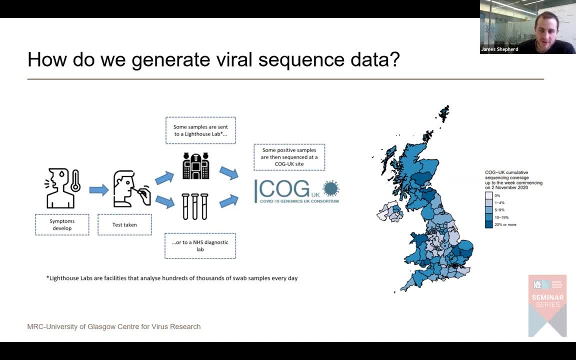 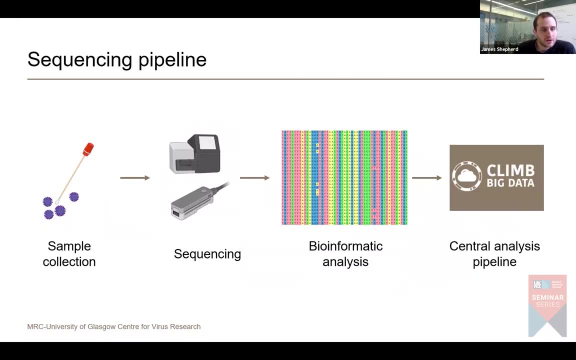 various locations across the UK. So this is kind of an unprecedented depth of genomic information we're getting from this pandemic. So once the swab with the virus and the genomic material arrives, the sample is inactivated here and the viral RNA is extracted. 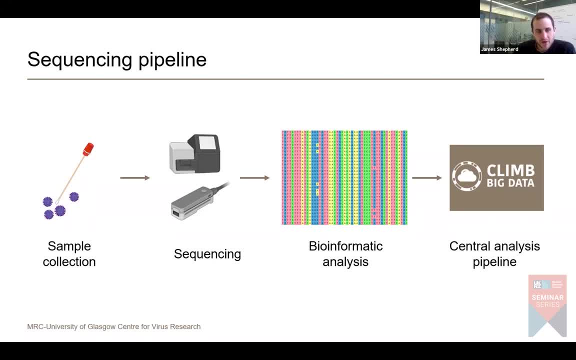 The nucleic acids in the virus are then fragmented and chopped up and run on these sequencing machines that generate the data as chunks of viral sequence, And these chunks then need to be assembled into the full 30 000 base pair long viral genome, and we do that by computational or bioinformatic methods here. 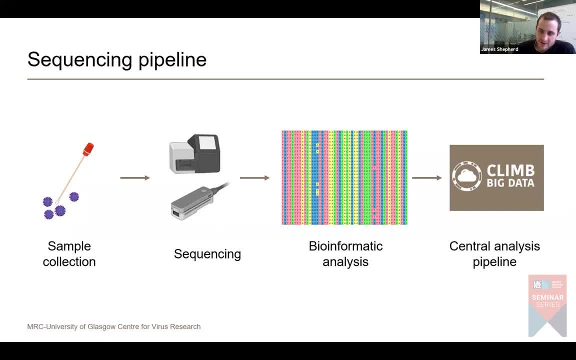 And then, once that's processing is finished, it gets submitted to a central computer cluster which is, I think, hosted in Birmingham and Cardiff and is also funded by MRSU funding. The computational pipeline there analyzes thousands of these sequences every day in parallel and then generates analysis that can 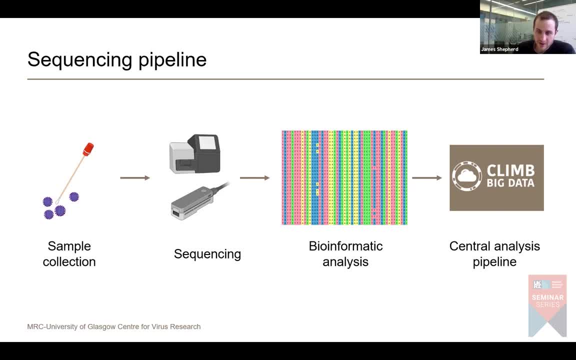 be fed back to public health agencies and NHS organizations and can be used for various scientific analysis. This whole process can be can be done in less than 24 hours if we need to get an answer very quickly about an IP or something like that, And it's important to note that there's 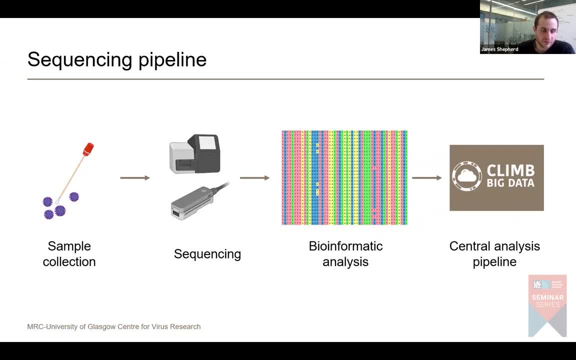 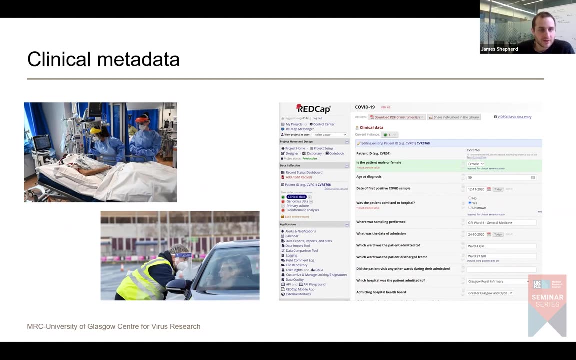 multiple people involved with various different skill sets, and right from the sample collection stage all the way up to this analysis pipeline, So a really collaborative effort to get this working. So, in addition to the virus genome, we need to get clinical data to put it into context and to 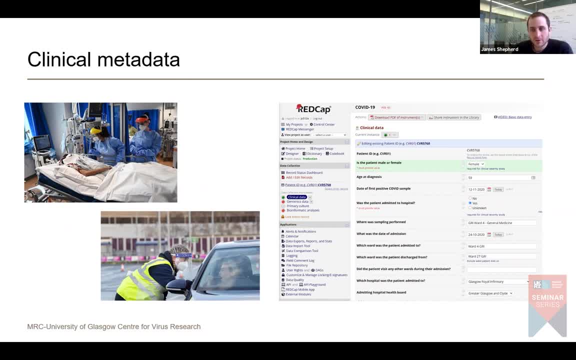 really get the most out of the information we're producing. So we want to be able to link the information we get from the genome to the individual patient. So we collect data on things like age, sex, the date we sampled, The sample that the swap was taken, things like travel, history and and in Glasgow we've gone a. 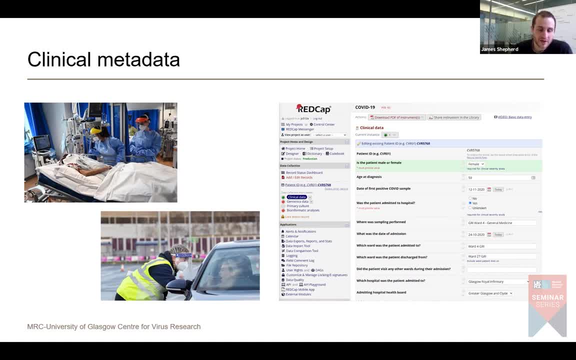 step further and we also are recording quite detailed information on patient outcomes. So some people will have a relatively mild illness, others have severe illness and be required to attend hospital and may even die. So we want to be able to look at determinants of that outcome in sequenced data. So we record that for every patient that we do. 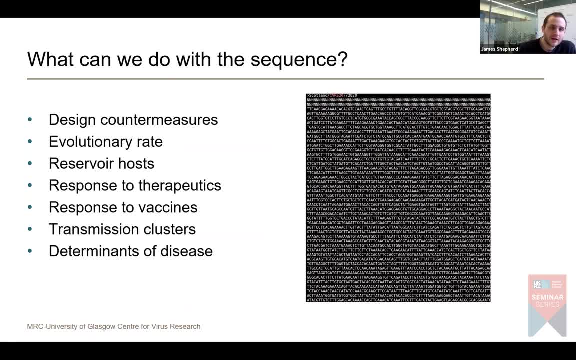 we get a sequence. for Once we have all these sequences, there's lots of things we can do, So we can use them to design countermeasures, such as vaccines and treatments for COVID. We can look at the evolutionary rate of the virus and how quickly it's evolving if we have lots of samples. 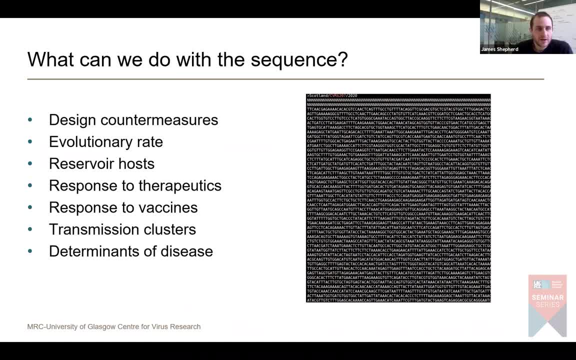 We can look at that and how it's spreading through populations. We can estimate what the reservoir hosts are. so how does it come from bats or pangolins? We can do that kind of analysis and we can look at the response to the virus genome and to therapeutics and vaccines. So do. 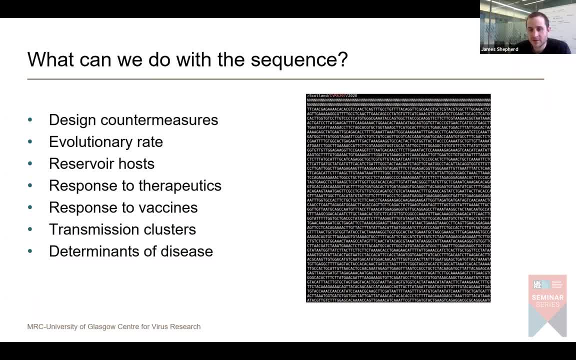 we see a change in the virus that's circulating when something like the vaccine is introduced, and does that have implications for whether or not the virus will continue to work? We can also use it to investigate transmission clusters and look at determinants of disease severity within the genome. So if someone has a particularly severe presentation, is there something? 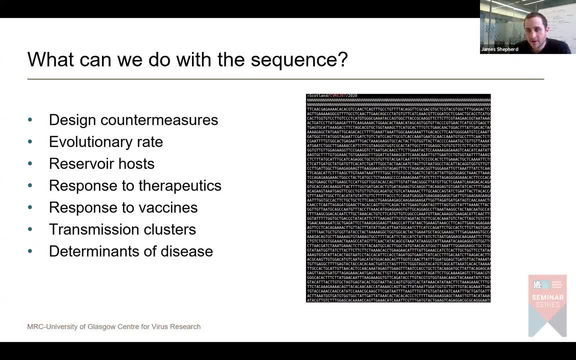 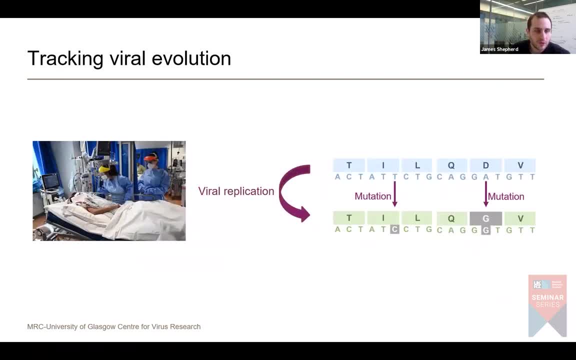 in that person's viral genome. that's going to tell us, gives us clues to why they've not done as well. So what we look for are changes in the virus as it replicates and spreads through the population. So every time the virus infects a person and replicates- and there's a possibility that it- 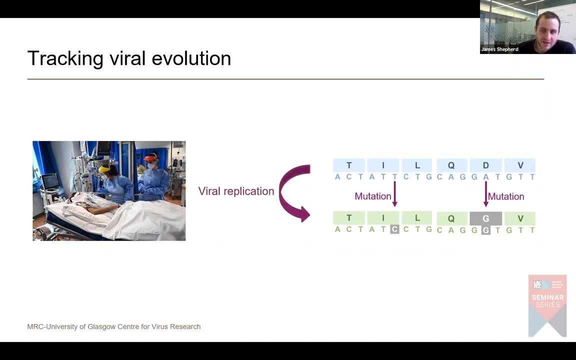 might make a mistake in copying its genome. If these mistakes are compatible with the virus continuing to be able to replicate and transmit, they become fixed in the genome and they become mutations. So here, if this person has a very severe transmission and they're not able to do that, 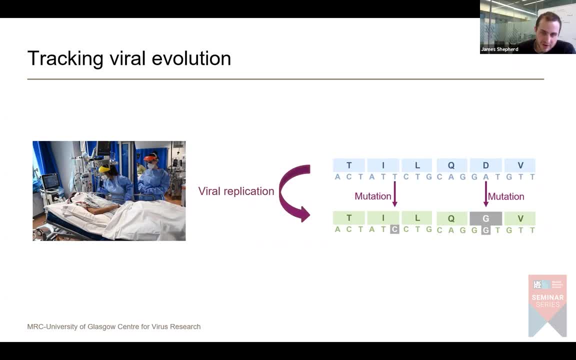 we can look at the gene sequence and see if there's any change in the gene sequence. So some mutations are usually in the gene sequence, but we can also look at the gene sequence of the person who's infected with this virus containing this particular genetic sequence which codes for 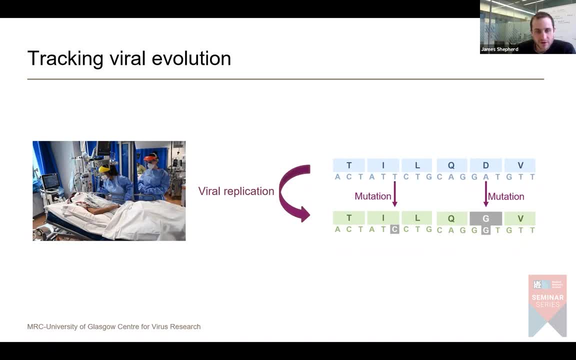 these amino acids. If we see a mutation in that, that will go on to be transmitted to the next person. Some mutations just change the genetic code itself, so the nucleotide sequence, but don't make a change with the protein sequence, Whereas other mutations may change the nucleosotide. 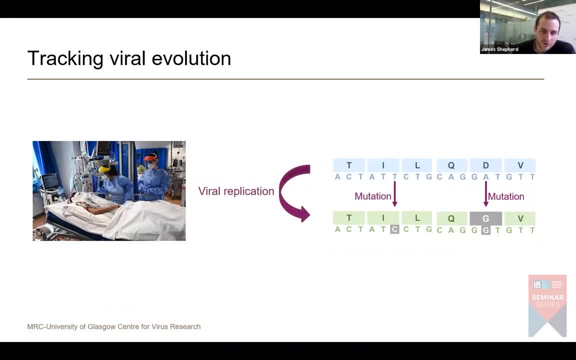 coded for. So some mutations are kind of silent, don't change the virus phenotypically. Others might change the protein sequence and change how that virus behaves. So we're looking for both of these mutations and we can use them in different ways. So understanding the genetic code can also 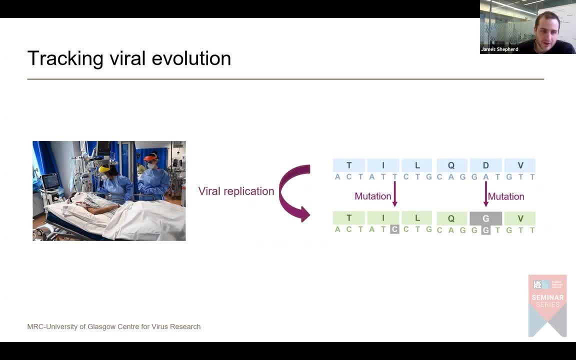 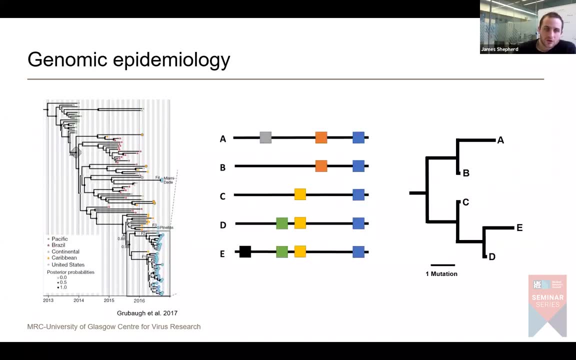 lead us to understand what changes in the protein we're seeing as the virus travels through populations. So because mutations can happen rapidly- so on an average twice a month we see a mutation in the SARS-CoV-2 genome- we can use them to reconstruct transmission networks. 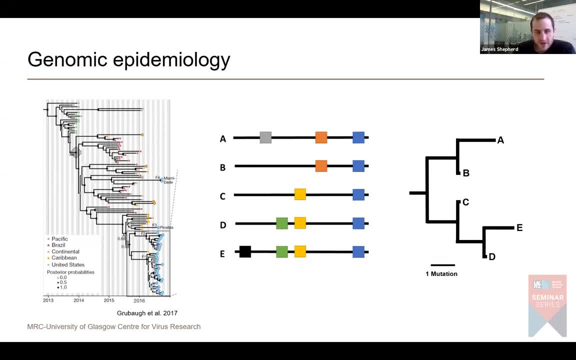 as the virus travels between different people. This is a technique called genomic epidemiology and it's previously been applied to other outbreaks such as Ebola or Lassa fever. This is an example of a fibromyalgia. This is a phylogeny from the Zika virus outbreak, and we build these phylogenies, which are essentially 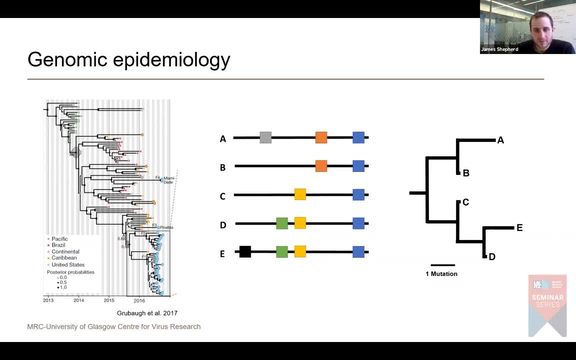 some evolutionary history of the virus by aligning viral sequences derived from multiple infected individuals to create this visual representation. So if you imagine that these five- A, B, C, D and E- are genome sequences from the virus from different individuals and the coloured squares represent, 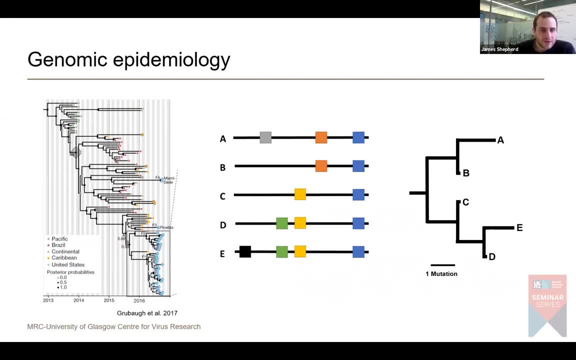 mutations. If we were to take sequences A and B, they both share these two blue mutation and this orange mutation. So when building the phylogeny, these two sequences and the virus from these two individuals would be grouped together and these little tips of the phylogeny represent those sequences. When you look at 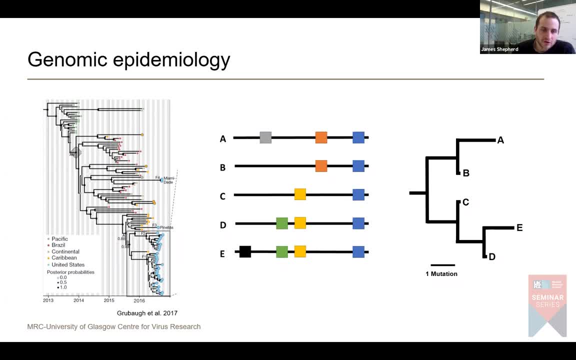 sequences C, D and E. they don't have the orange mutations, but they all do share this yellow mutation, so they would be grouped together on the tree If we were to take sequences A and B. they both share these two blue mutations and the coloured squares represent 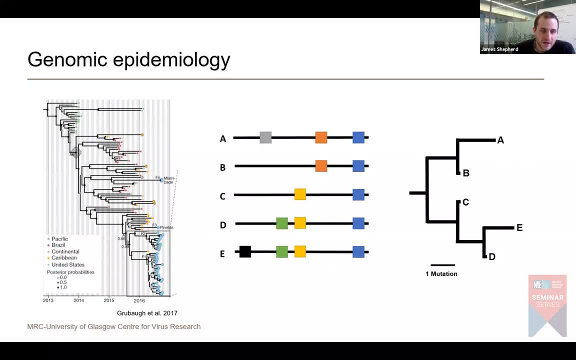 And then, going on from that, D and E have this green mutation and they would cluster together. So then we can infer that the virus from person E, because it shares these mutations with D, is most likely related to this virus D, Whereas it's less likely to be related to virus A, which doesn't share these mutations and has these additional orange mutations. 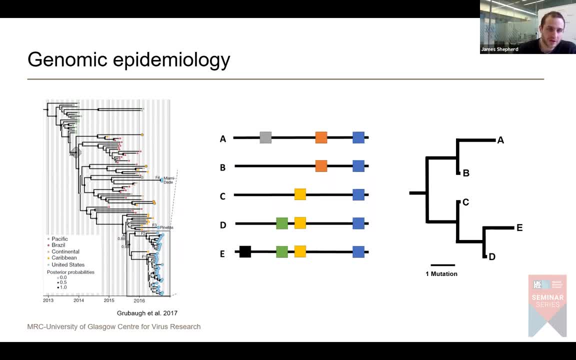 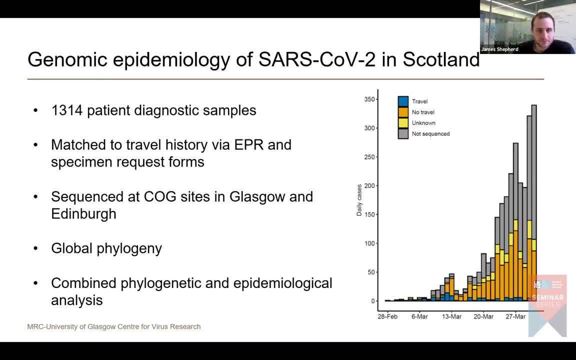 And that's how we build the phylogeny that we do on a larger scale. So we wanted to apply this genomic epidemiology method to investigate how SARS-CoV-2 entered Scotland. We had managed to sequence quite a high proportion of the cases in the first wave. 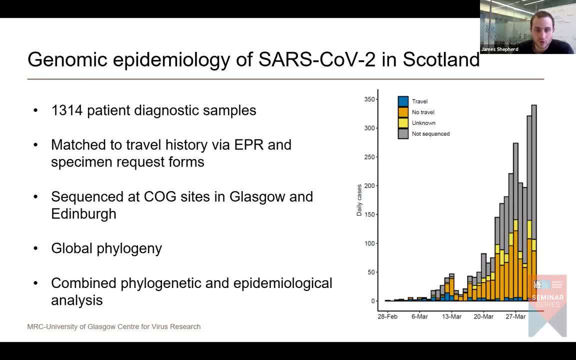 So we had roughly 50% of all the PCR positive results. we had a whole genome sequence for And you can see, in the first wave in Scotland we kind of started at the end of February And then by the beginning of April or the end of March we were experiencing about 350 PCR positive cases every day. 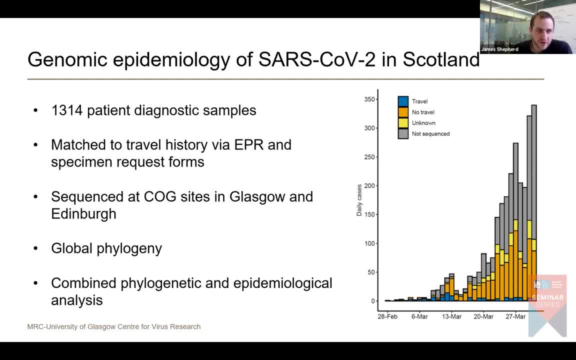 And we had quite detailed information via electronic patient records and special specimen request forms on whether or not these individuals were trampled or not. We had information on the dates of sampling, So we performed a combined analysis using the genome sequences that we generated the dates of infection. 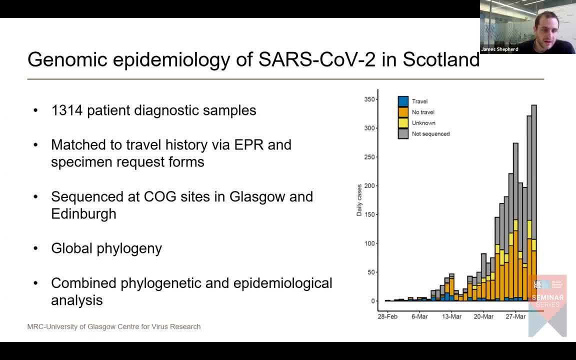 We had epidemiological data that we had from individuals, such as travel history, and we generated a large phylogeny using all the genome sequences available to us of SARS-CoV-2 leading up until the end of March, And then we did an analysis of that. 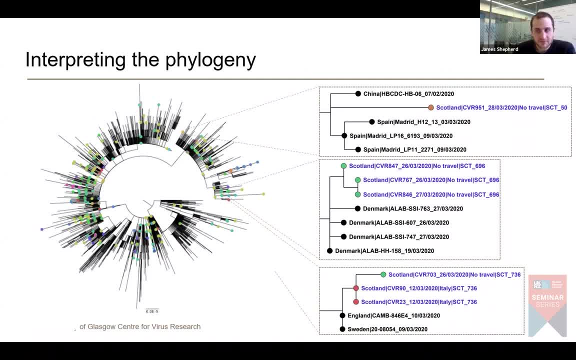 So we generated an enormous phylogeny which had an excessive 20,000 sequences and it's far too big to display properly on a PowerPoint slide or really on any digital slide. And we did that until the end of March. And then we added our Scottish sequences on top of that. 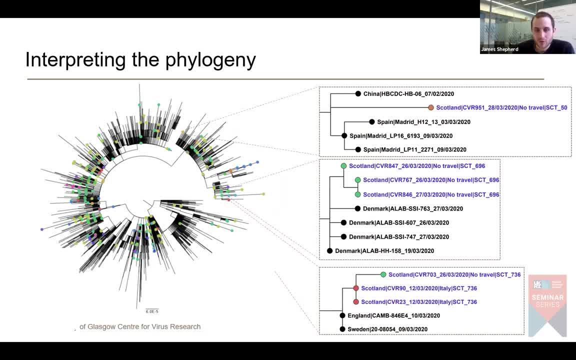 So our 1,300 Scottish sequences, And we looked at where the Scottish sequences were popping up in the phylogeny and looked at how they really were in relation to other sequences from the evolutionary tree from around the world And where they clustered, where they emerged. 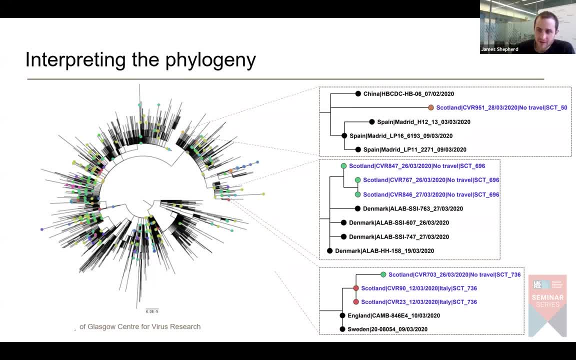 We from From the other sequences. We call that an introduction into Scotland. so we're identifying a unique virus with its own mutations that's been introduced into Scotland from the wider pool of circulating viruses throughout the world. We term these introductions transmission limits. Scottish transmission lineages. 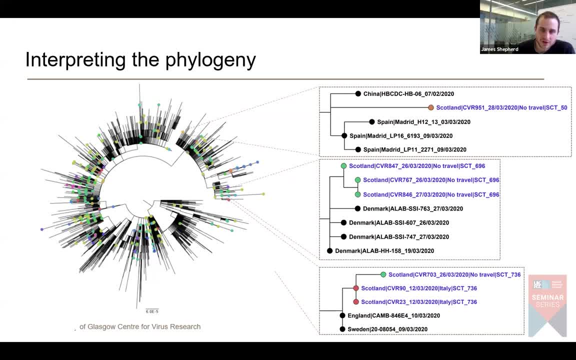 So we had some where we had evidence of one individual bringing the virus into Scotland or being infected, but no onward travel. And then we had other examples of lineages where an individual may have brought the virus back and it's resulted in onward infection in other individuals in Scotland. 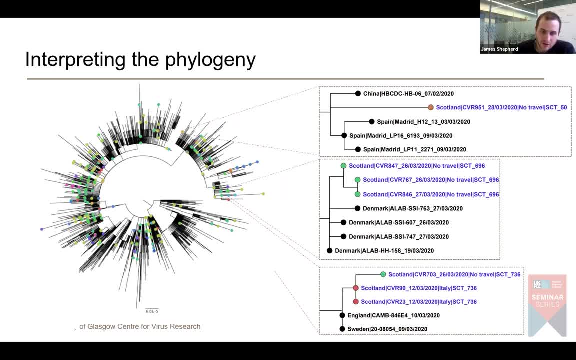 And then we had some cases where we had a good travel history of the individual. So, for example, these viruses were sampled from individuals that had travelled to Italy and were seen, based on the genomic data, evidence of onward transmission from them to Scotland. So we used a computational process. 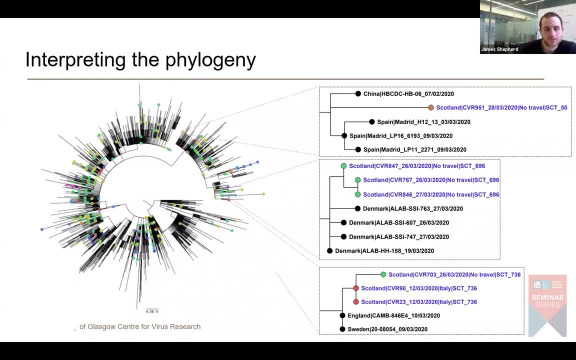 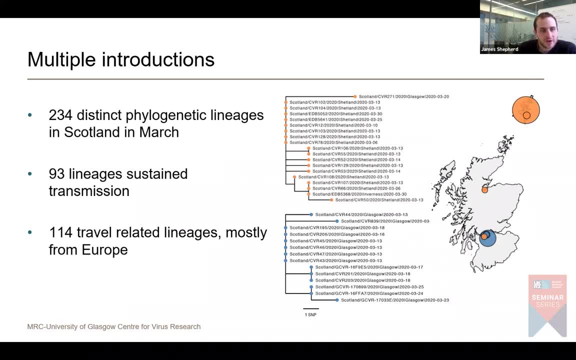 to go through this enormous tree and pick these out, And what we saw was that there were 234 distinct biogenetic lineages in Scotland in March, So we think 234 viral introductions into the country. 93 of these resulted in large transmission lineages with multiple sequences. 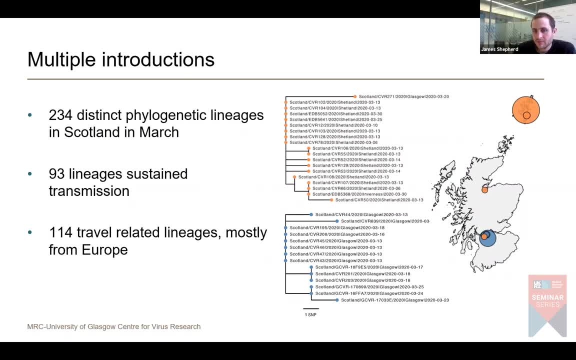 And we could annotate geographical data onto these And we could annotate geographical data onto the tree and combine that And some of these looked quite geographically clustered. So, for example, there was a outbreak in Shetland and the genomics showed that all these cases were related to an introduction to Shetland and one introduction lineage in Scotland. 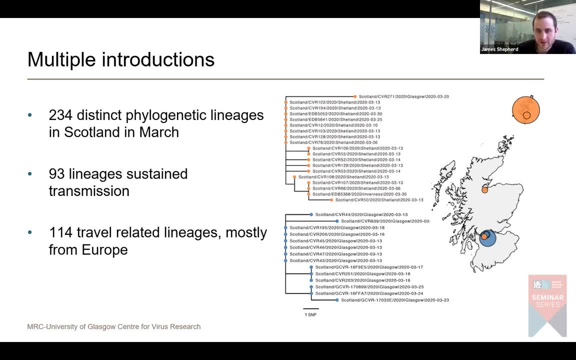 So, for example, the gold represents Shetland. We were also able to identify other cases that were linked to this cluster that didn't reside in Shetland, And there were other larger clusters which were linked by genomics But were more distributed across Scotland. 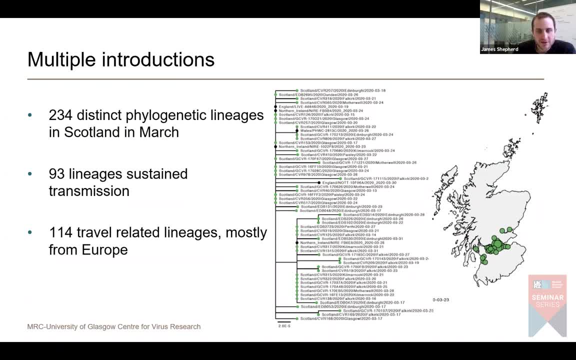 And again, the genomic sequencing allowed us to link these cases together and understand how the transmission of COVID and show that this was the result of one viral introduction. So, 114 of these biogenetic lineages, we were able to determine a link, a known link, to travel, so a travel related case. 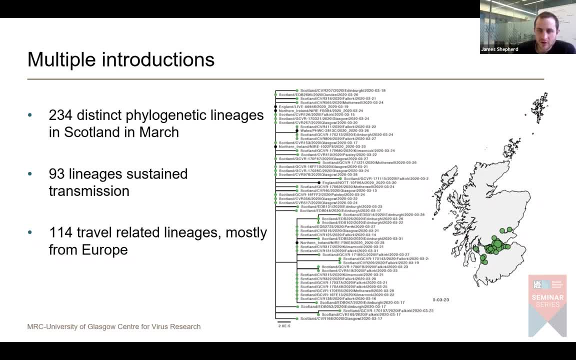 But for the other ones we weren't able to add To identify any known link to travel. So that suggested to us that people were traveling back to Scotland despite the virus not being identified by the screening measures that were put in place at the time to test symptomatic conditions. 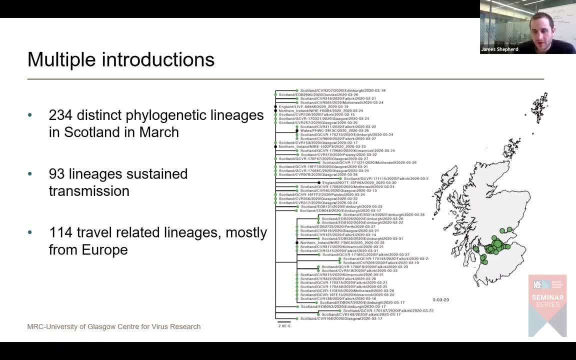 The other interesting thing we found was that most of the travel was from Europe and that there was hardly any introductions of the virus from China. When we looked at the phylogeny, we also found that there wasn't really any genomic evidence of introductions directly from China. 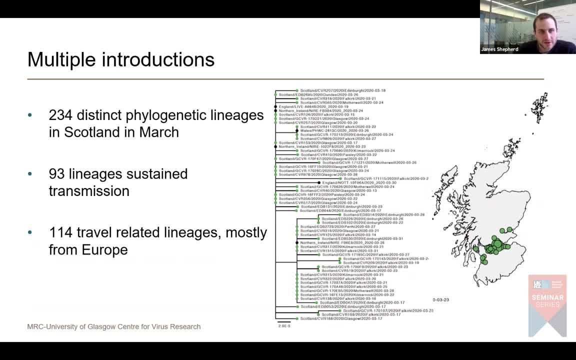 So we think that might reflect that there was good travel restrictions related to China around this time But there wasn't such good messaging of travel or restriction of travel around Europe. So it kind of shows that the outbreak that we have here in Scotland and the wider UK is really a European outbreak. 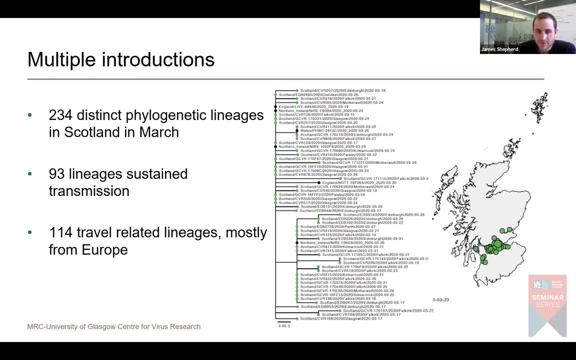 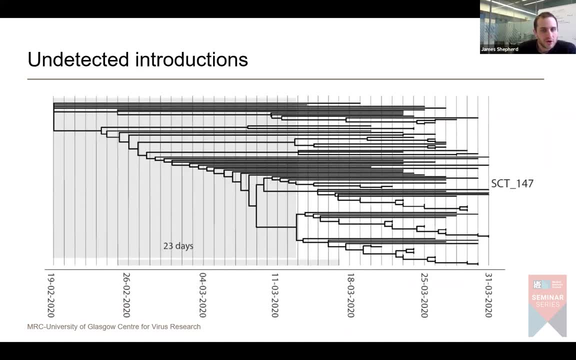 And it isn't directly related to the outbreak in China. So, as far as this goes, it was via other European countries mostly. And we can also use a special type of phylogeny called a time scaled phylogeny, Where the x-axis, instead of representing evolutionary distance, represents time. 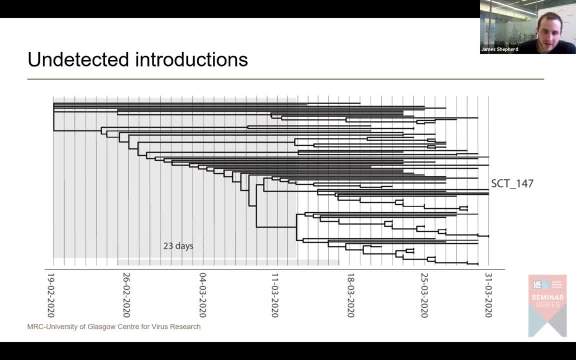 And we apply this to all of our lineages and we're able to estimate when we think the virus was first introduced into Scotland. Looking back at them all, we think that the virus first came to Scotland. There's a common ancestor of all these sequences in Scotland: around a couple of weeks before it was initially detected and suggested it was circulating. 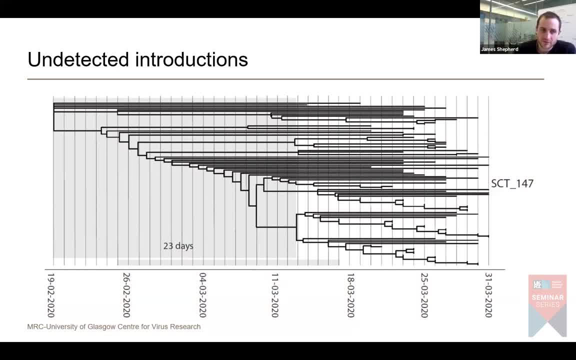 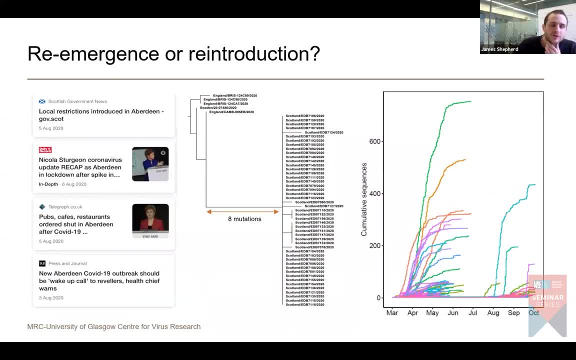 And evading detection for several weeks before we saw the first case. So once we understand the lineages that we have circulating, we can pull them up over the next few months, And that's what we did, using genomic sequencing of positive cases, assigning each sequence to one of the lineages. 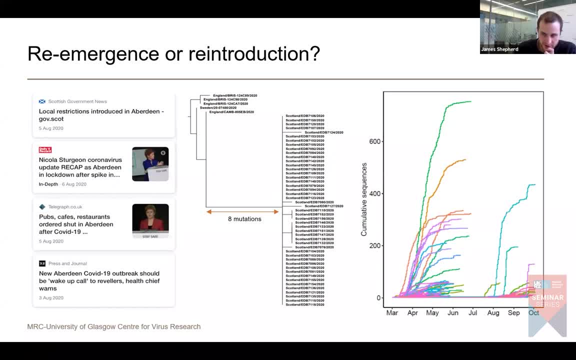 And we can also identify new viral lineages when they appear. So, thinking back now to August, the city of Aberdeen was placed in lockdown because there was a large outbreak there And we did some sequencing of those cases and we were able to show that the virus that was introduced represented a new lineage that we hadn't seen in Scotland yet. 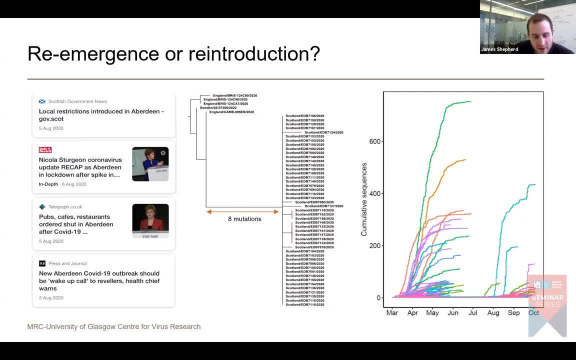 So this wasn't a case that spread from the first wave that had popped up again in Aberdeen and caused this outbreak. This was something that had been introduced from abroad, And you can tell that because it was so different to anything else we'd seen in the country before. 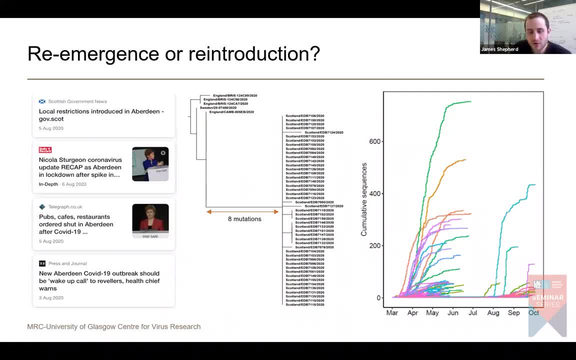 It was a big one. So that gave us a warning shot as to the role travel might play in driving the second wave And what we see when we plot the size of the lineages on the plot. So if we look at the time, there's time on the x-axis here, and on the y-axis we have the cumulative sequences. 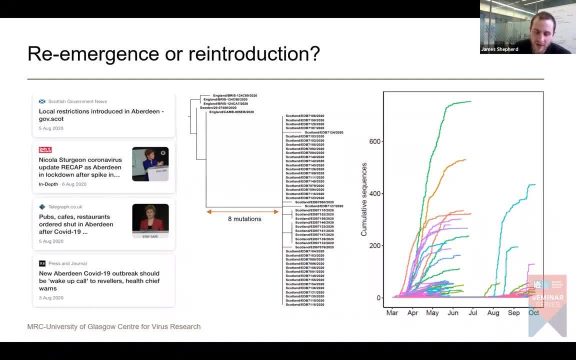 And each line represents a lineage. You see, in the first wave the lineages grow very rapidly, But as lockdown occurs the rate of growth slows And they kind of peter out in the summer as lockdown takes its course And they actually start to die out. 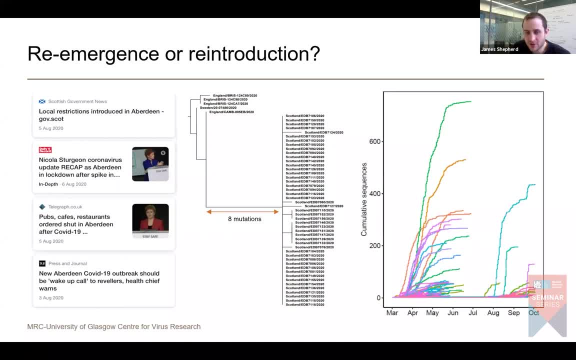 Not many of the lineages actually sustain transmission in Scotland over the summer. What we see when the second wave begins at the start of August is that these are new lineages that are being introduced from the country, Not something that we've ever seen before in Scotland. 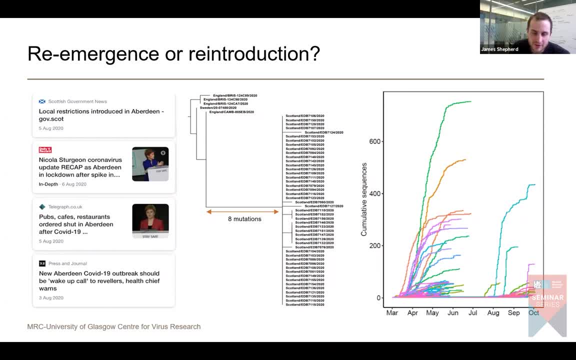 And these are related to travel. So the genomic data here is showing us two things. It's showing us that the first lockdown was really very effective in reducing transmission And we almost managed to eliminate the virus in Scotland, And we see these lineages just dying out. 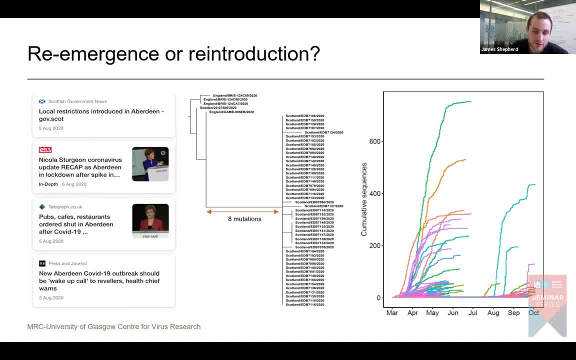 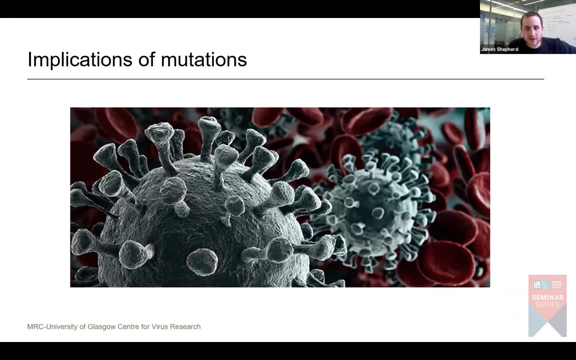 But once things open up, introductions of new lineages from abroad start to fuel the epidemic, And that's kind of how we got to the situation we are in now with another lockdown. So, given how it's quite topical at the moment, I'm just going to talk a bit about how some of the ways the genomic data has been used, identifying the significance of various mutations that have arisen during the pandemic. 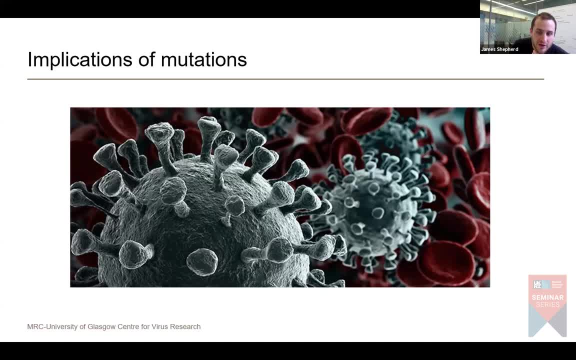 So most of the mutations that we have gathered a lot of interest recently are directed at mutations in the spike protein, which is this protrusion you see from the virus whenever you see it photographed or on television or in the news- something This spike is the one that we're interested in. 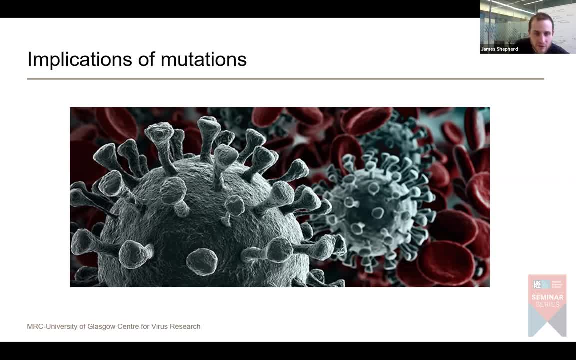 And it's an important protein because it mediates entry into our cells. So when the coronavirus infects someone, it gains access by the spike binding onto our cells, And it's a spike binding onto a receptor in human cells called ACE2 receptor. 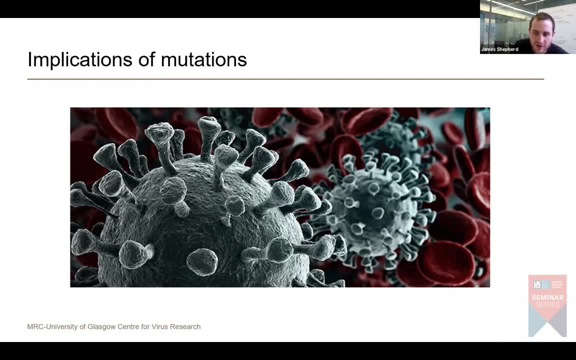 It's also important because the spike is a major target for our immune system And, specifically, it's a target for proteins that our bodies produce in response to vaccination or infection, called antibodies. And these antibodies that are produced in response to a vaccine or infection bind to the spike protein, block it and they stop the virus being able to enter our cells because it's covered in antibodies. 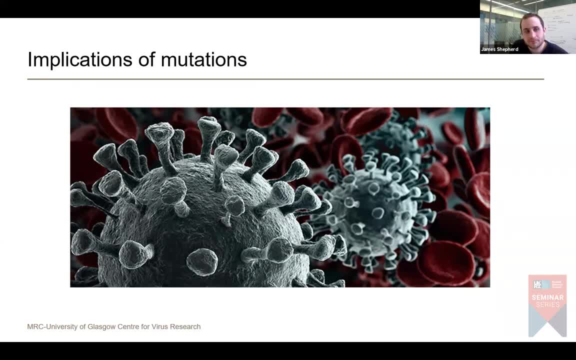 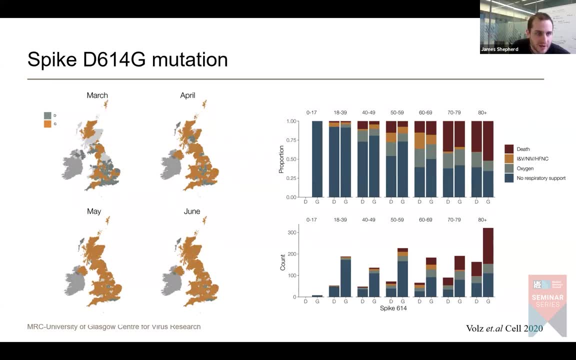 So it's an important protein for the virus And it's also important because the spike is a major target for these reasons. So back in the summer there was evidence that a particular mutation in spike called D614G was coming to high frequency in the UK. So mutations are described by their position in the protein. So the spike protein is 120, sorry, 1,270- amino acids long. So this nomenclature here suggests that the D amino acid at position 614 in spike has been replaced by a gene. 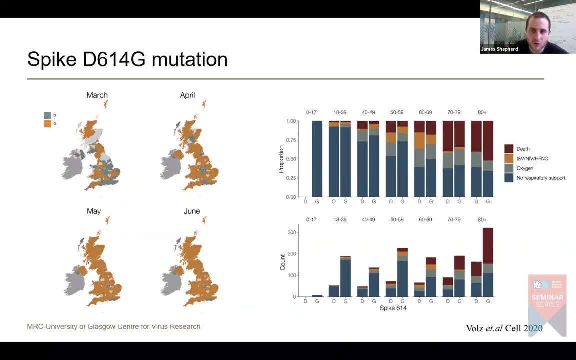 So if you hear these names, like N501Y or whatever that means, there's been a replacement in amino acid at that particular site. So in March at this site about half the isolates we saw had this D amino acid And the other half had this G, which is D stands for aspartate and G is glycine. 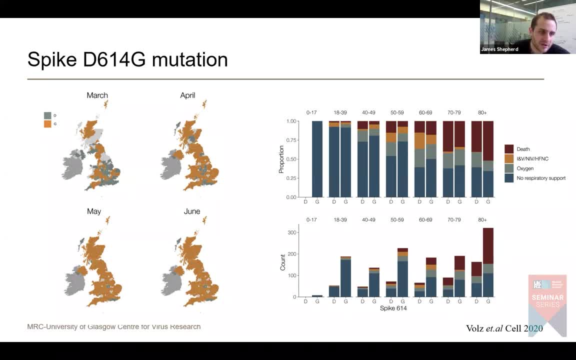 So two different amino acids. What we saw as the months went on is that the Ds were completely replaced almost by the G. So people started wondering: is the G giving the virus an advantage in making it spread better, And is that having an effect on clinical outcome or transmission? 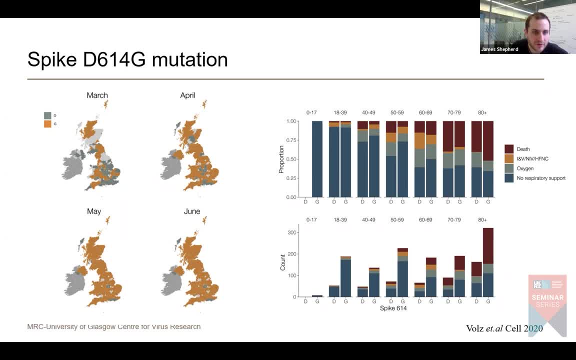 So because we had we linked all the sequences we've done back in the summer, which is we've done back to the clinical outcome of patients, we were able to take a good look at this. So we were able to stratify all our patients based on whether or not they had the D or the G. at this position, 614. 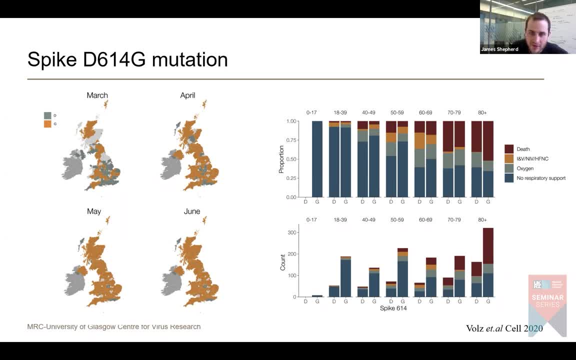 And we were able to look back and see what their clinical outcome would be. So have they died? Have they required intubation and ventilation or high-flow oxygen? Have they required hospitalization for oxygen, Or did they get on fine and not require any respiratory support? 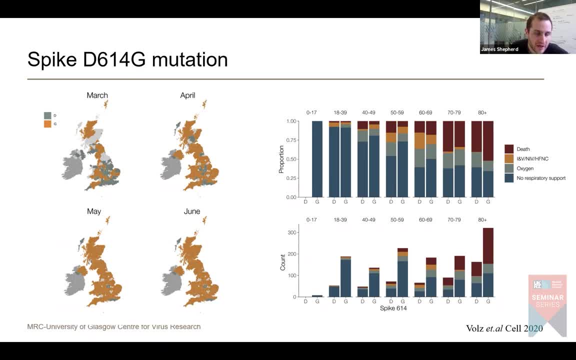 So we did an analysis of this and it showed that there was no effect of this mutation clinically, So patients weren't becoming more sick because of it, And you can see in this graph that these are the age groups. As you go up the age groups, the main determinant of doing badly and having a poor outcome is actually age. 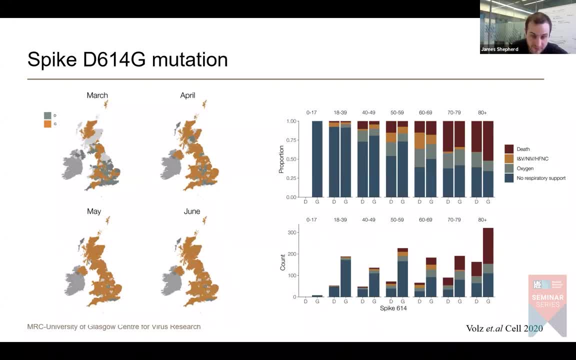 That's quite clear in this visualization that age is the main thing, But there wasn't any significant difference between the two groups with Ds, So that was quite reassuring. This wasn't making anyone more sick, But it did appear that the virus spread slightly better if it had the G. 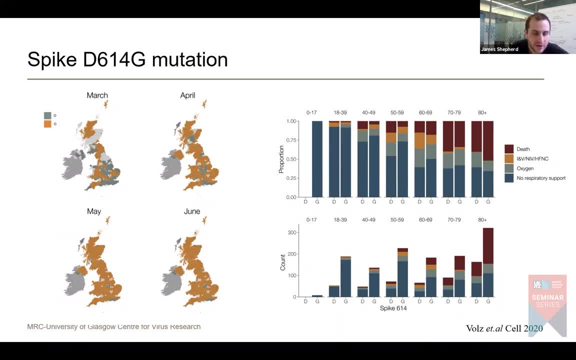 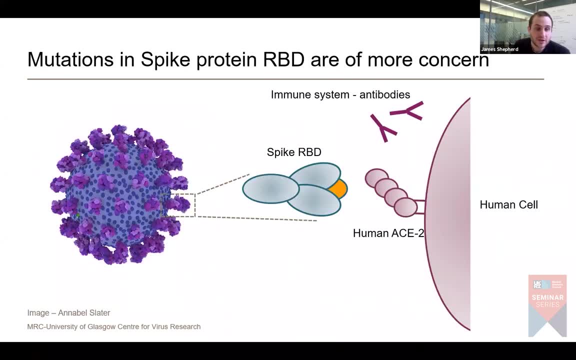 So this is an example of how we can link clinical outcomes back to a genome data to answer questions. Some of the recent mutations that have arisen in the spike protein are of more concern, And there's a particular part of the spike protein called the receptor binding domain. 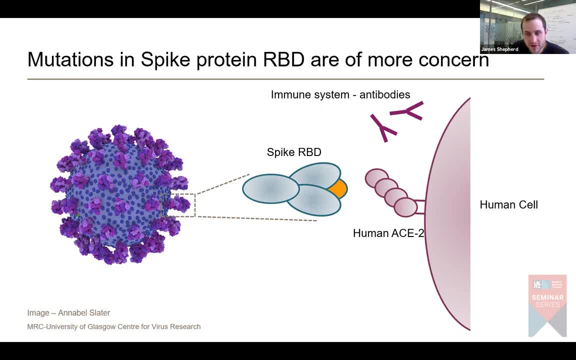 That's been a focus of a lot of attention And this particular domain is important for two reasons. This is a part of the spike protein where the virus binds on to our human cells by binding to this human ACE2 receptor, So it's very important with regards to entry. 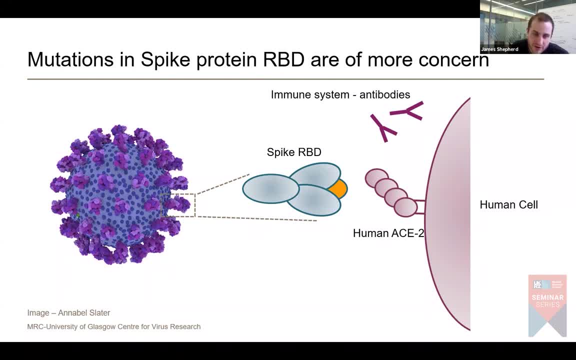 So we're very interested in any changes in this part that might result in it entering the cells better or efficiently, or less efficiently, And it's also the most important part of the spike protein for recognition by these proteins I've mentioned before, which are induced by infection or vaccination, called antibodies. 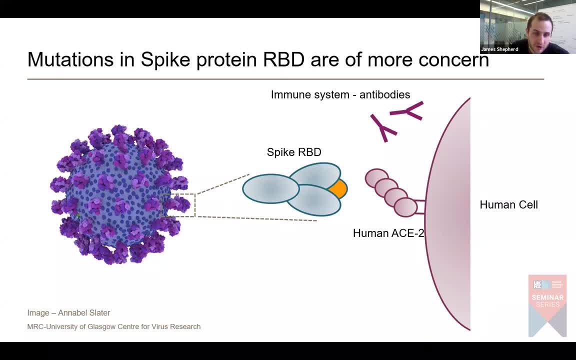 So antibodies- the most important antibodies our body produces- bind to this receptor binding domain. So any changes here might alter entry into cells And it might also mean that the virus that has a change here might be able to escape recognition by antibodies. So that would obviously be a concern. 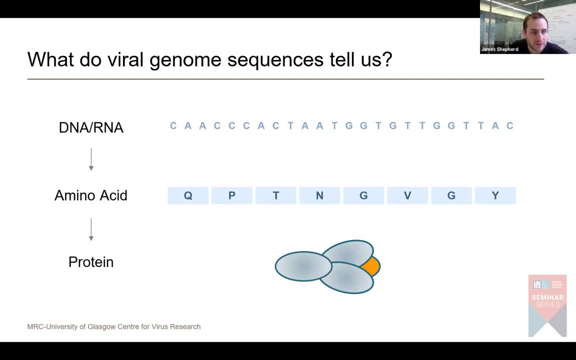 So, just going back to the flow of information, if you remember that we have DNA or RNA in the case of the virus, which codes for amino acids, which then can code for the protein, So like our spike protein with its receptor binding, And if there's a mutation in a certain part of the genetic code that might lead to an amino acid change. 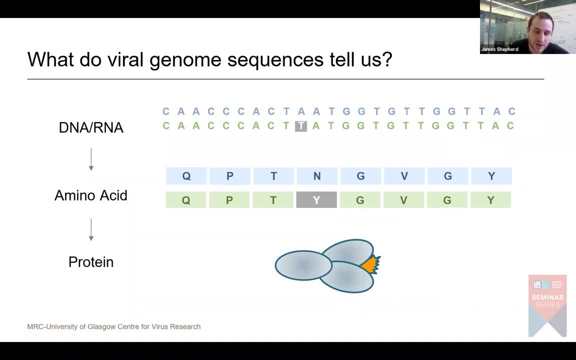 And that might lead to a change in the protein, So a change in shape of the protein that might change its function or mean it's not as well recognized by antibodies. This is what we've seen with the variant that emerged in Southeast England just before Christmas and was responsible for the new lockdown. 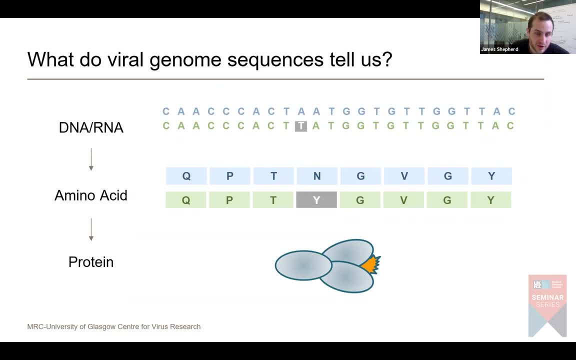 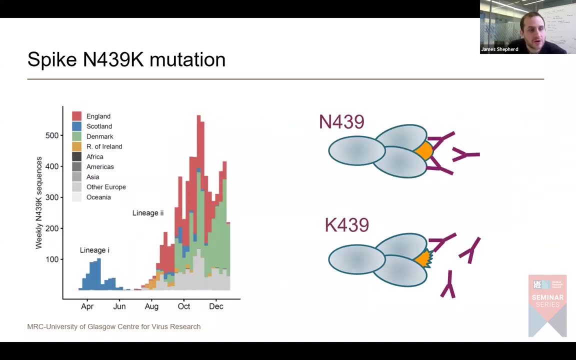 There was a change, an A to a T in the code for the spike protein. It's changed an amino acid which has probably changed the shape of this receptor binding domain and led to it spreading more quickly. So we had a bit of experience with this because we saw a similar change in Scotland back in April in spike, again in the receptor binding domain at position 039.. 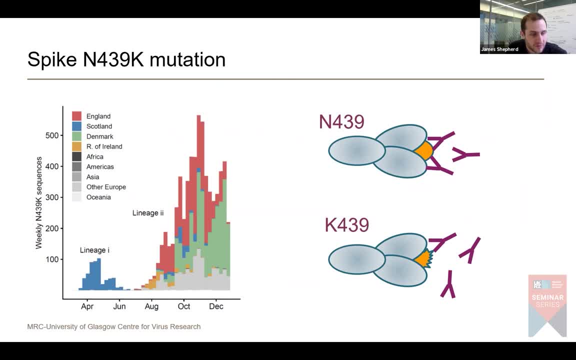 And this emerged and spread in Scotland, caused this lineage here, which reached quite high frequency but was eliminated because we did a lockdown. What we've seen is that this mutation has occurred again in several other lineages which would spread in England, Wales, Ireland and various other parts of Europe. 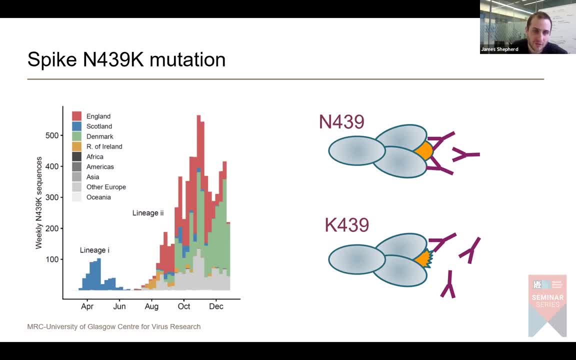 And so we, because we had identified this by sequencing, we could look at this in the lab. And so we went into the laboratory and did antibody binding assays, looking at the two different types, So the N, so the wild type, at 439, and then also the K, so the mutant, at 439.. 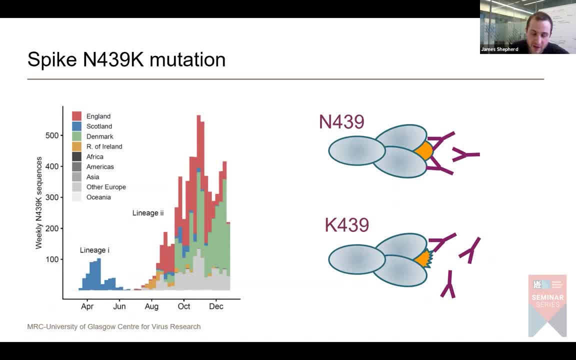 What we found was that the mutated form didn't bind to antibodies as well, But it didn't lead to any worse infection and it didn't lead to any increased spread of this mutant, So it just meant that people's antibodies didn't bind as well. 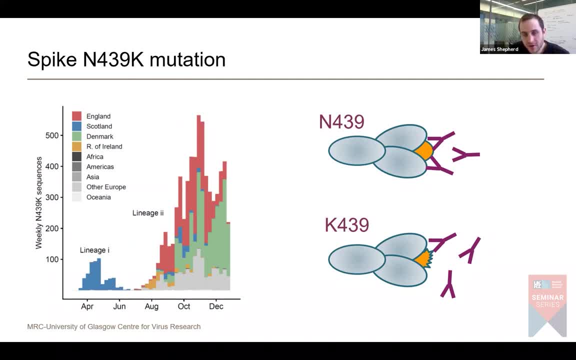 So further work is going on at the moment to see if that will also be the case with vaccines. So the concern is because the vaccine contains the code of this variant. if people are infected with this variant, the vaccine might not work as well. 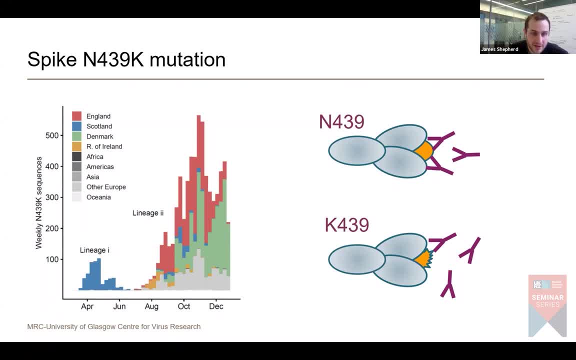 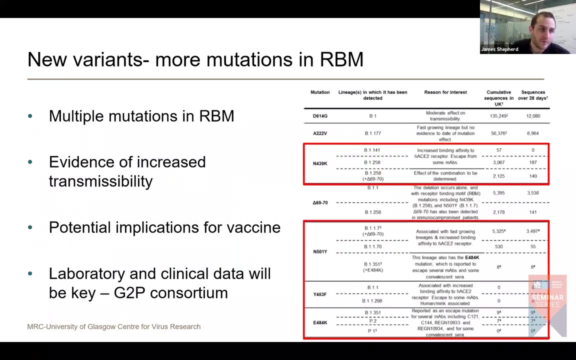 So we're going to study in the laboratory and also in the real world once we start vaccinating people and monitoring what viruses any people who have been vaccinated become infected with are going to be what really tells us as to whether or not this is significant. 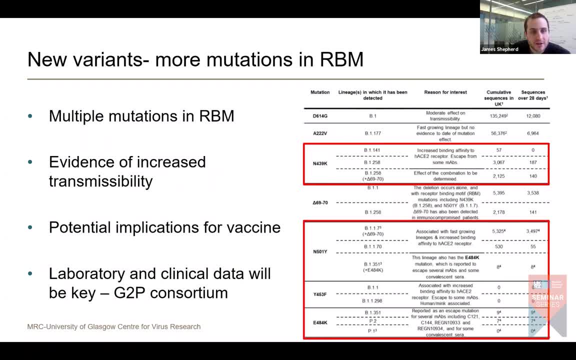 And something that a lot of people are concerned about are these new mutations in the receptor binding motif. So when we looked at N439K, there was a moderate reduction in antibody binding. It's not something that we're hugely worried about, But these other lineages have arisen. 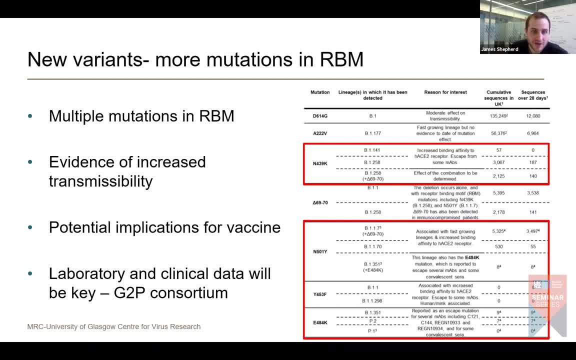 So there's the lineage that caused Christmas to be cancelled essentially, which has this N501Y mutation, And then there's other mutations which have occurred in Brazil and South Africa. So that's why we should travel bans against these countries, And it's not because we know that there's definitely going to be an impact on efficacy of the vaccine. 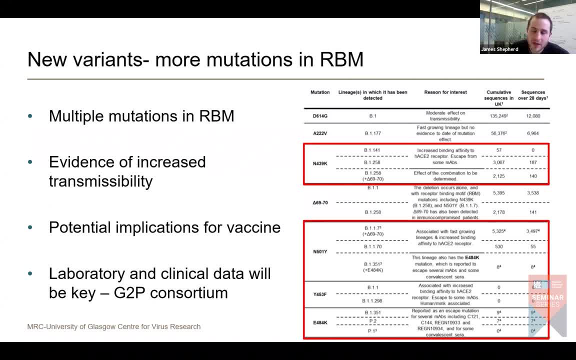 But it's basically being very careful because we don't want these spreading here, And there's evidence that some of them might be able to spread better than the current variants, similar to the one we saw over Christmas, So more work is going into this. 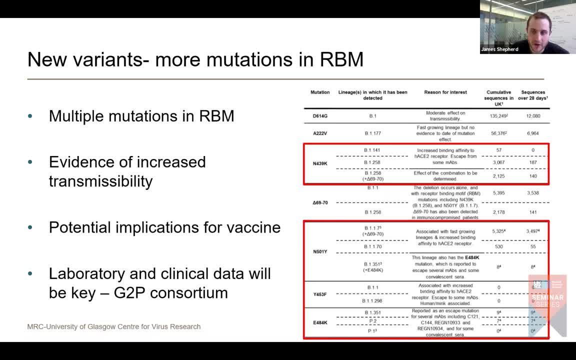 And there's just been funding from UKRI for a consortium to look at these changes rapidly in the laboratory. It's called the Genotype to Phenotype Consortium. But CROG-UK will still be important going forward in identifying these, identifying where they're emerging, how fast they're spreading and feeding into laboratory and clinical studies. 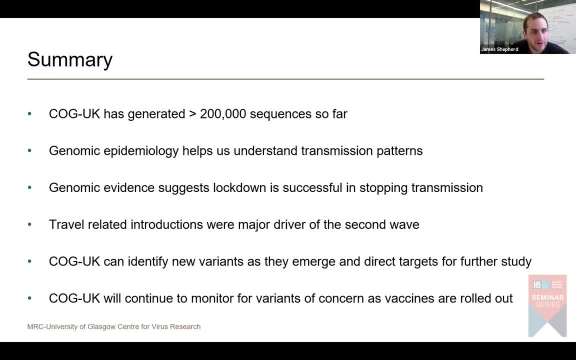 So, in summary, that was just a fairly broad overview of what we've been doing. CROG-UK has been really successful in generating a really good understanding of the genomic patterns of COVID and identifying mutations that have emerged as the epidemic's gone on. 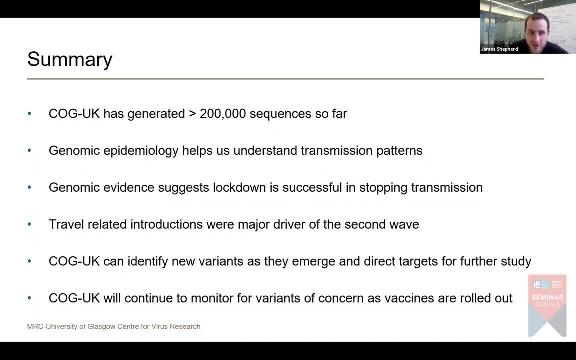 We can understand transmission patterns with genomic epidemiology showing that lockdown is successful in stopping transmissions. It's demonstrated the role of travel related to COVID. It's demonstrated the role of travel related to COVID. It's demonstrated the role of travel related to COVID. 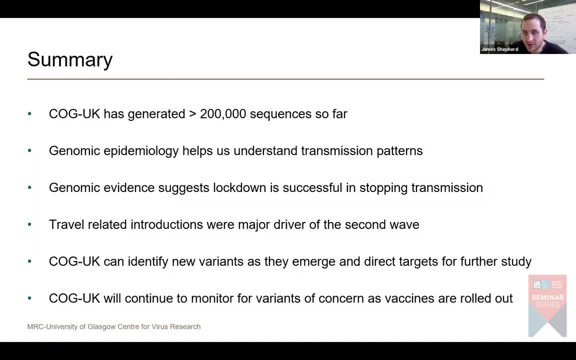 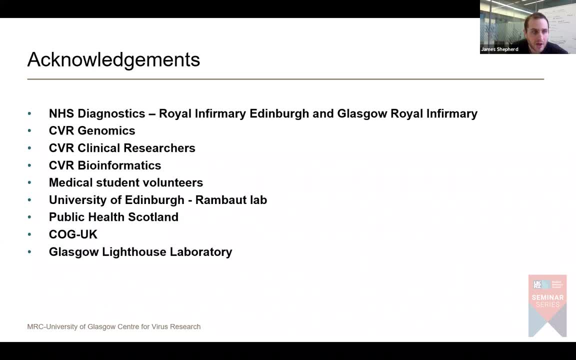 So we've been looking at those introductions which we think are the major drivers of the second wave, And CROG-UK will continue to look for new variants as they emerge and as vaccines are rolled out. And these are just some acknowledgements. 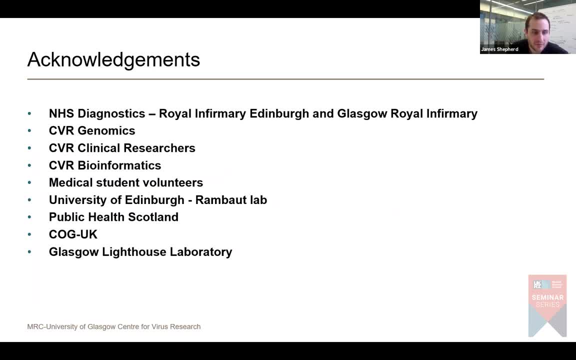 but there's just an enormous amount of people who have collaborated on this and it's been really- I guess it's been really- inspiring to work in this way where people have been so enormously collaborative and worked really hard. you know, haven't had much recognition for that, but then